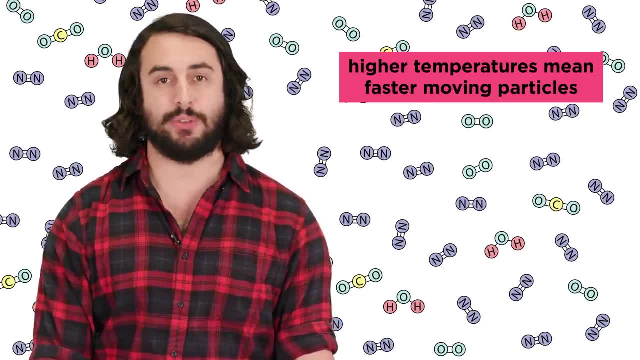 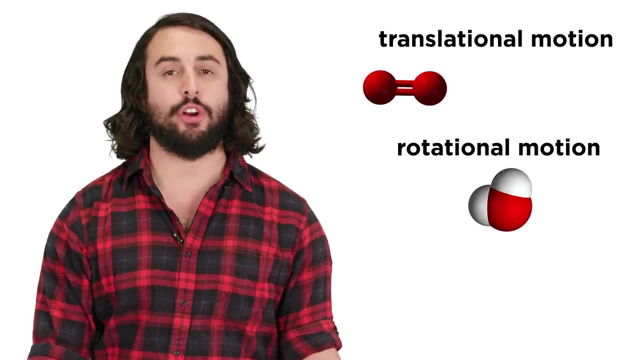 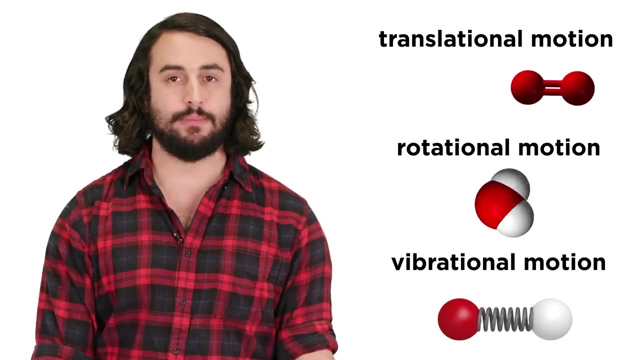 So higher temperatures simply mean faster moving particles. This kinetic energy of motion is distributed amongst translational or side-to-side motion, rotational or spinning motion and vibrational motion. where the covalent bonds in a molecule bend and stretch, Heat will flow from hot objects to cool objects, because as the particles move they will impart. 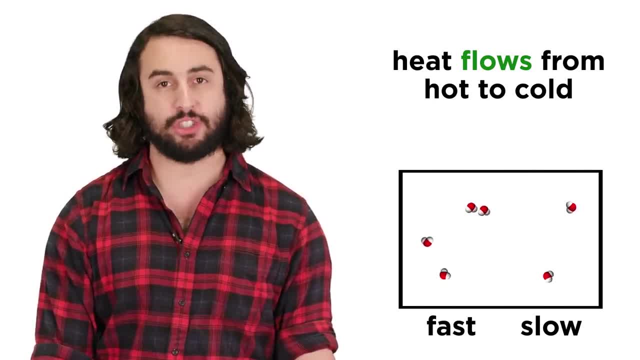 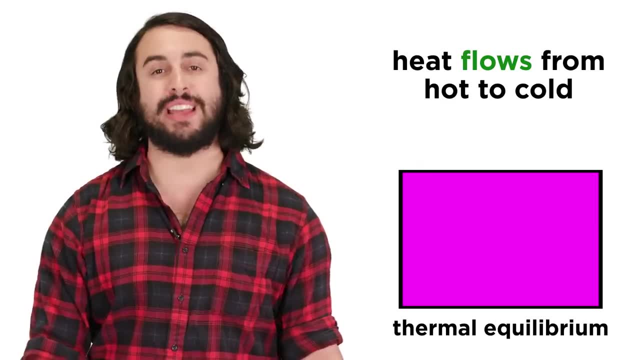 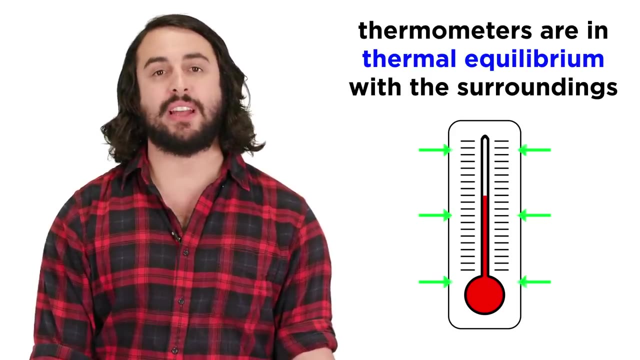 some of their kinetic energy onto other particles through collisions. This will continue to occur until the whole system is at the same temperature in a state called thermal equilibrium. This is how thermometers measure temperature. The environment will be in contact with the thermometer and flow into the thermometer. 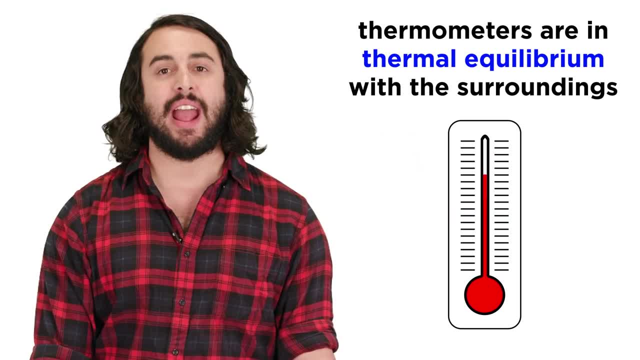 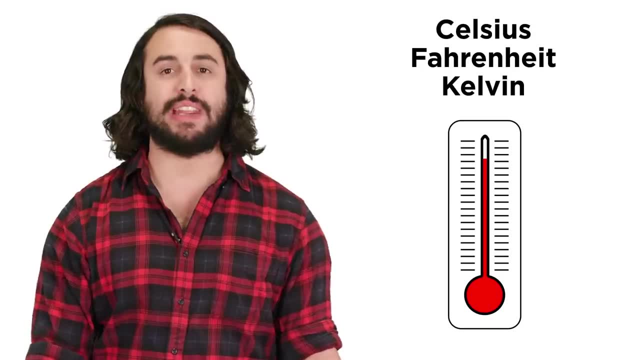 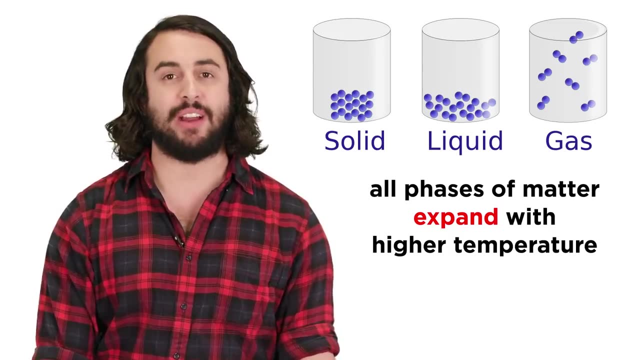 fluid, causing the atoms to gain kinetic energy, and the column will expand until it is in thermal equilibrium with the environment, thus allowing us to read the temperature in one of our man-made units. We must bear in mind that all phases of matter expand with higher temperature, whether solid. 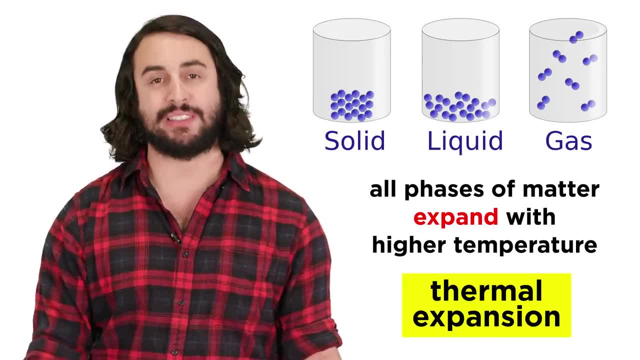 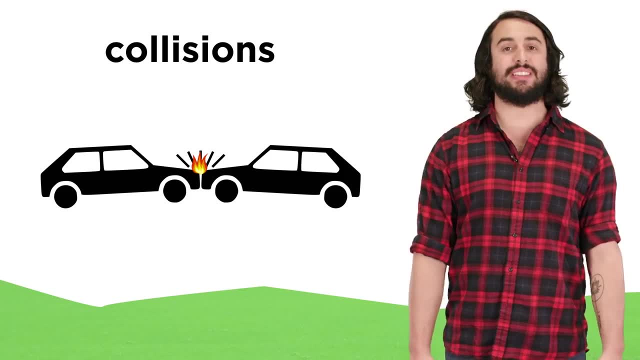 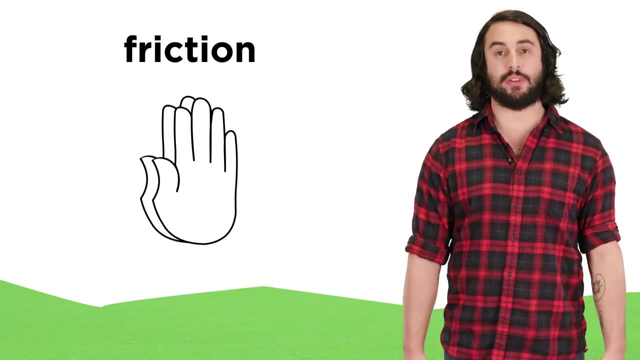 liquid or gas. This phenomenon is called thermal expansion. Energy is transferred as heat in a wide variety of processes. When a collision occurs, there is usually some heat generated. Friction can cause heat as well, which is why your hands warm up when you rub them together. 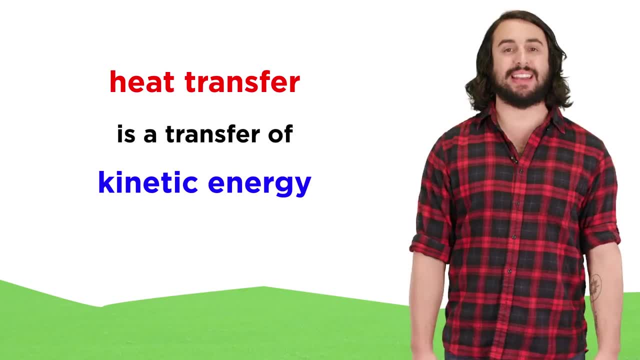 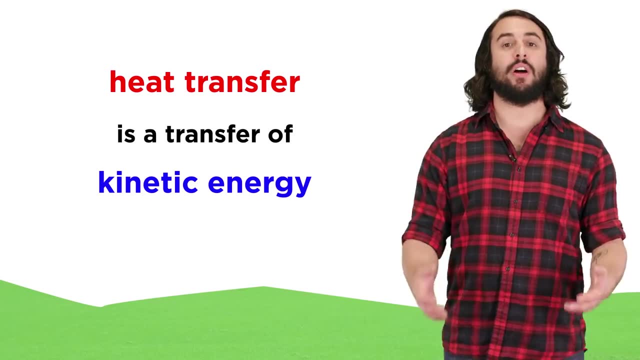 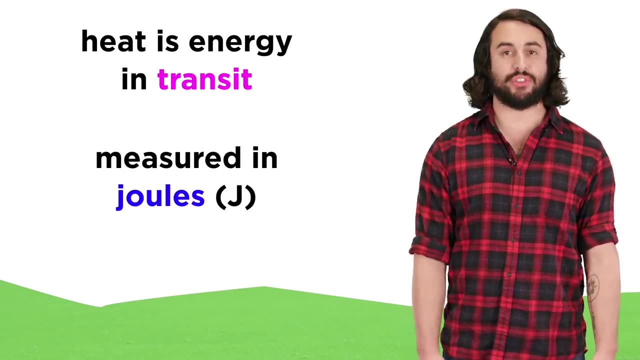 vigorously. In each case, we are considering the kinetic energy of the particles and the transfer of some of this energy to other particles as the definitions of heat and heat transfer. Heat is therefore a kind of energy in transit and will be measured in joules, just like a. 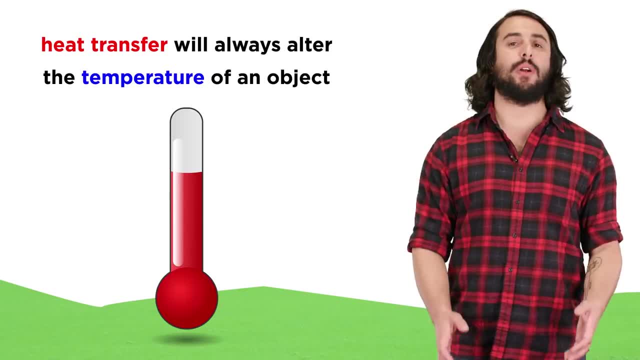 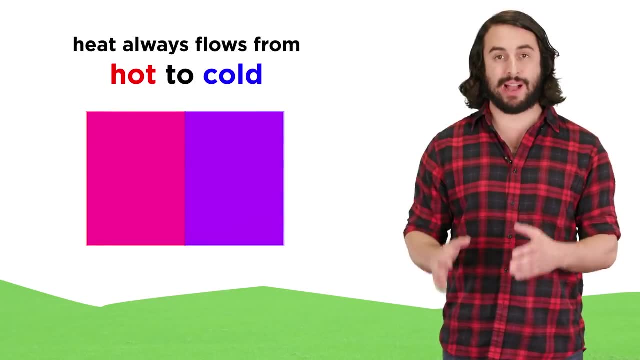 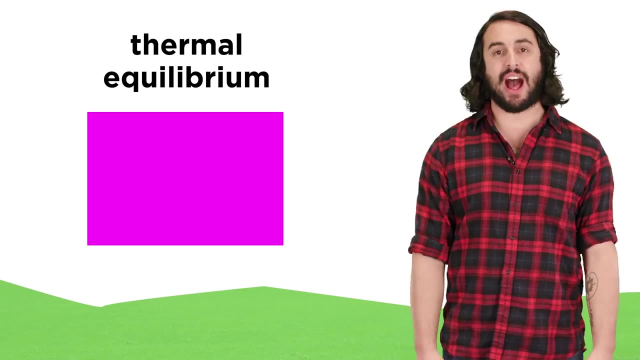 particle, just like any other kind of energy. Furthermore, the transfer of heat energy will always alter the temperature of an object, as heat will always flow from the higher temperature object to the lower temperature object until thermal equilibrium is reached. This is why hot objects feel hot and cold objects feel cold. because a hot cup of coffee. 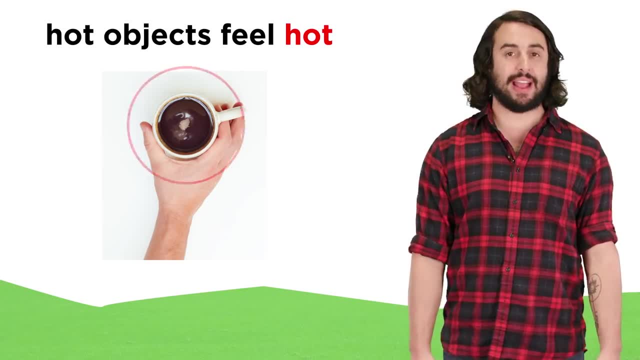 which is hotter than your hand, will transfer heat into your hand, while a cold piece of ice, which is colder than your hand, will cause heat to flow into your hand. This is why hot objects feel hot and cold objects feel cold. because a hot cup of coffee. 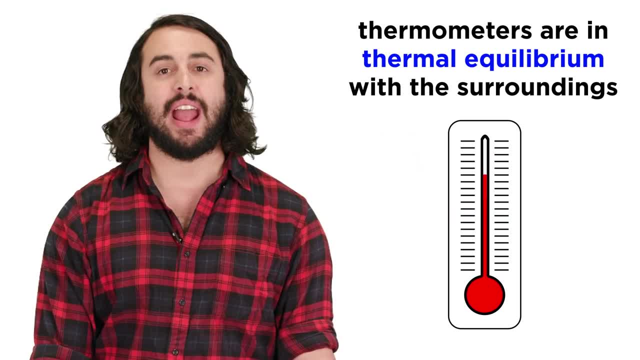 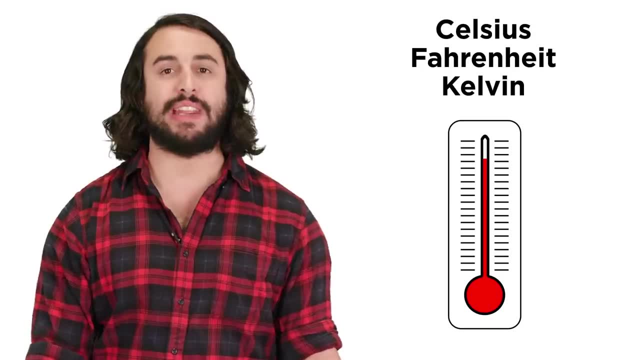 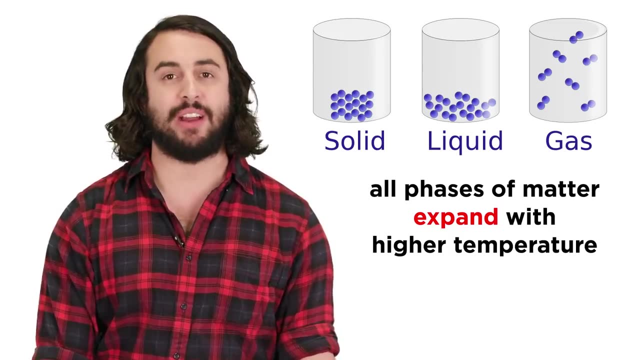 fluid, causing the atoms to gain kinetic energy, and the column will expand until it is in thermal equilibrium with the environment, thus allowing us to read the temperature in one of our man-made units. We must bear in mind that all phases of matter expand with higher temperature, whether solid. 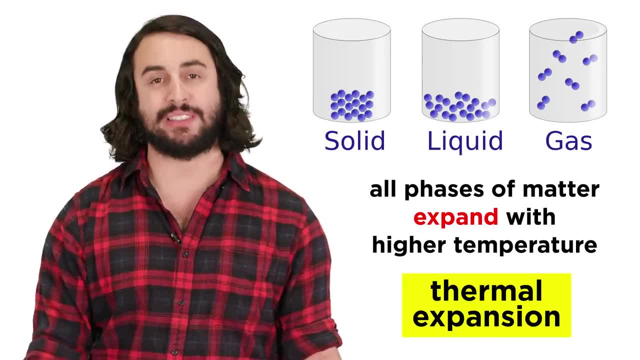 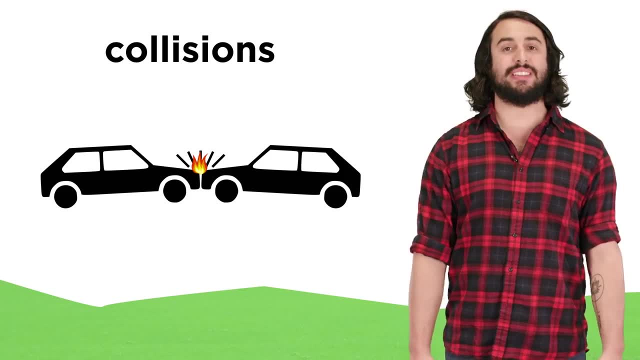 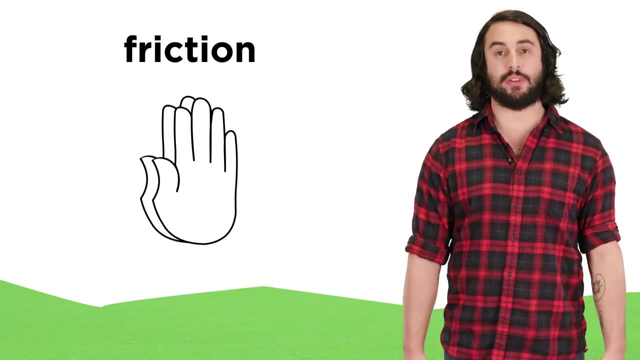 liquid or gas. This phenomenon is called thermal expansion. Energy is transferred as heat in a wide variety of processes. When a collision occurs, there is usually some heat generated. Friction can cause heat as well, which is why your hands warm up when you rub them together. 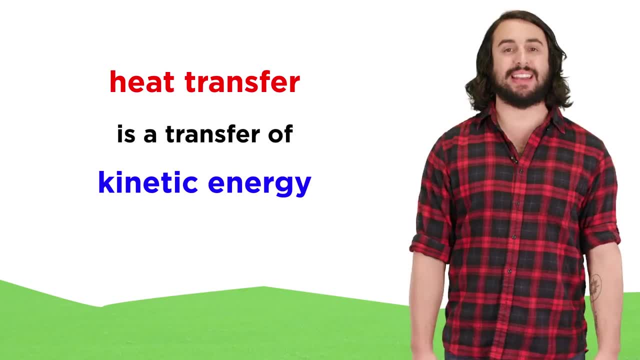 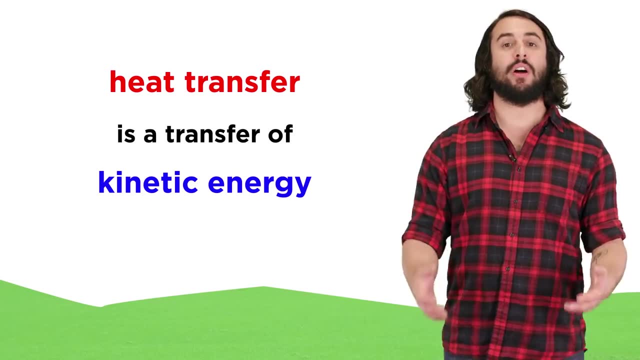 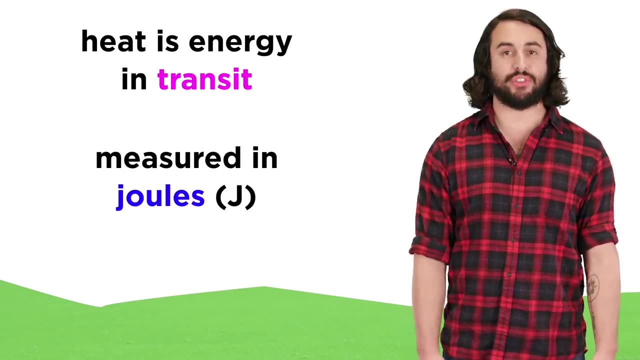 vigorously. In each case, we are considering the kinetic energy of the particles and the transfer of some of this energy to other particles as the definitions of heat and heat transfer. Heat is therefore a kind of energy in transit and will be measured in joules, just like a. 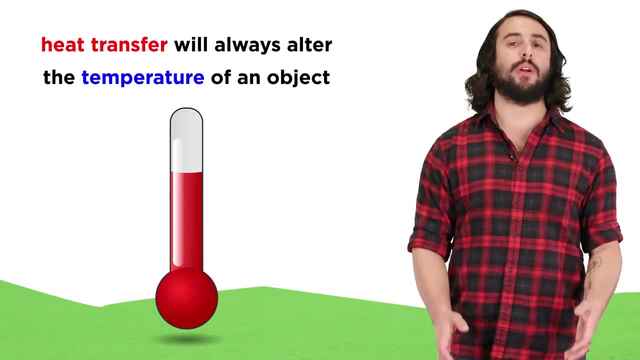 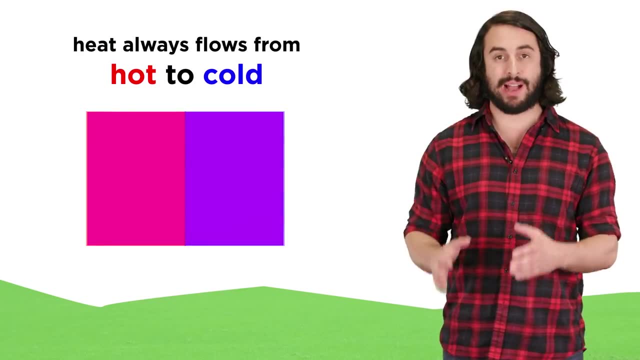 glass of water. This is just like any other kind of energy. Furthermore, the transfer of heat energy will always alter the temperature of an object, as heat will always flow from the higher temperature object to the lower temperature object until thermal equilibrium is reached. 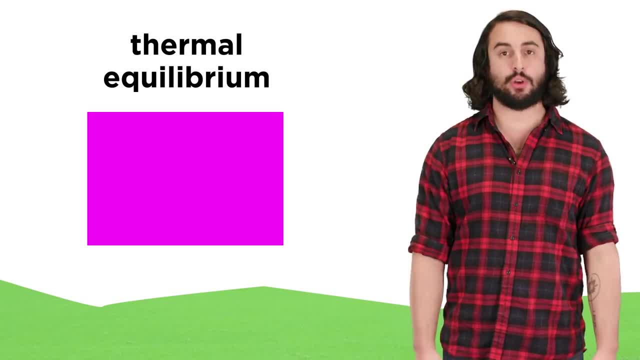 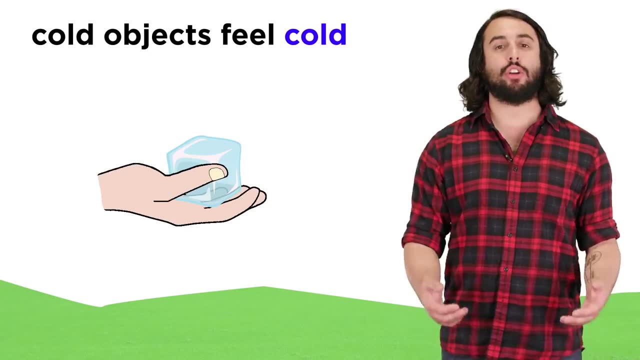 This is why hot objects feel hot and cold objects feel cold, because a hot cup of coffee, which is hotter than your hand, will transfer heat into your hand, while a cold piece of ice, which is colder than your hand, will cause heat. 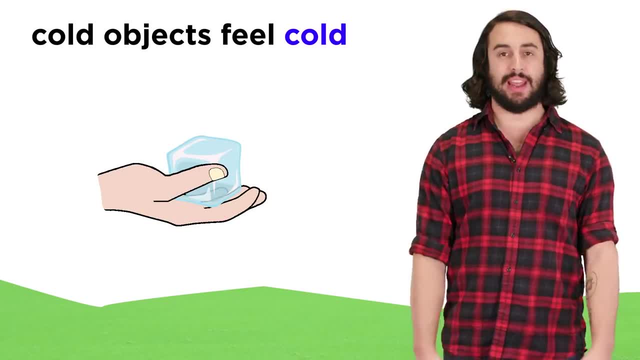 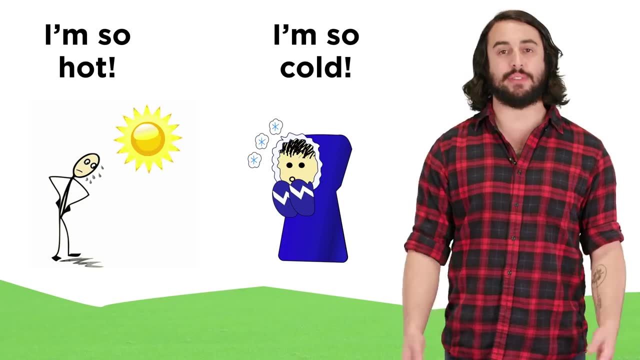 Heat will transfer heat into your hand, while a cold piece of ice which is colder than your hand will cause heat to be transferred out of your hand and into the ice. These events produce the hot and cold sensations we feel in our day to day lives. 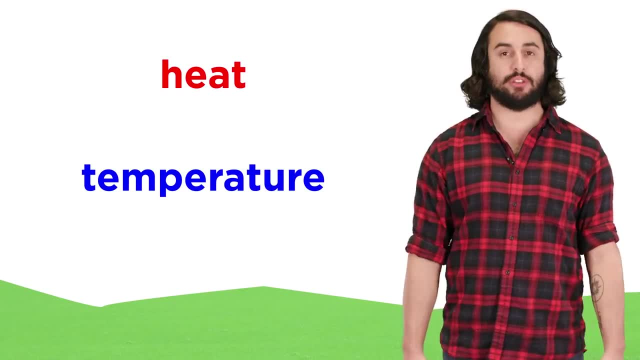 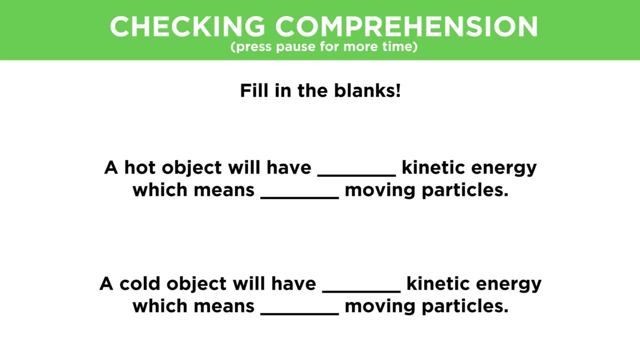 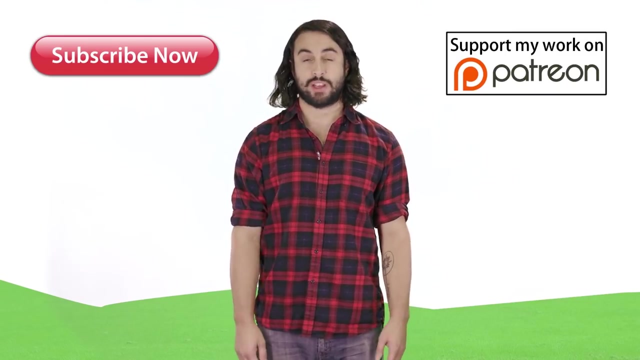 Now that we better understand heat and temperature, let's check comprehension. Thanks for watching, guys. subscribe to my channel for more tutorials. support me on patreon so I can keep making content and, as always, feel free to email me. professordaveexplains. 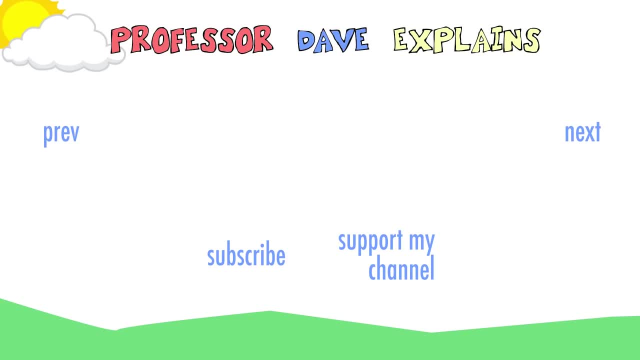 at gmail dot com. I'll see you in the next video. bye. 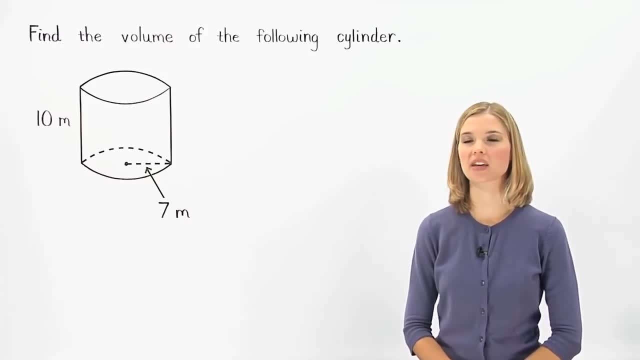 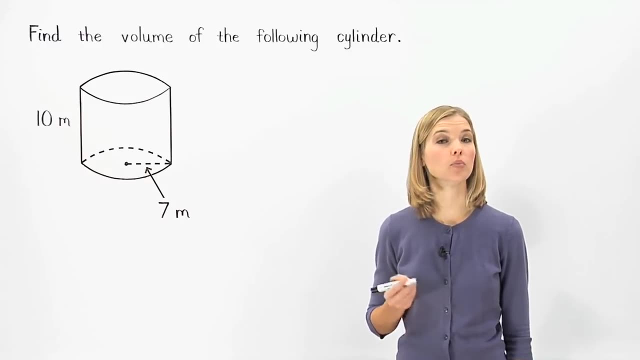 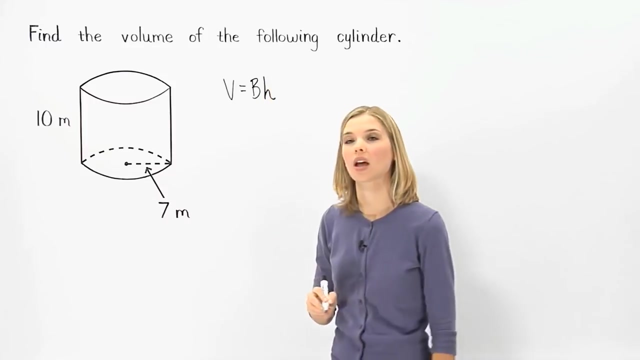 In this example, we're asked to find the volume of the given cylinder. To find the volume of a cylinder, we use the same formula that we use to find the volume of a prism. Volume equals area of the base, times height. Notice, however, that the base of a cylinder is a circle. 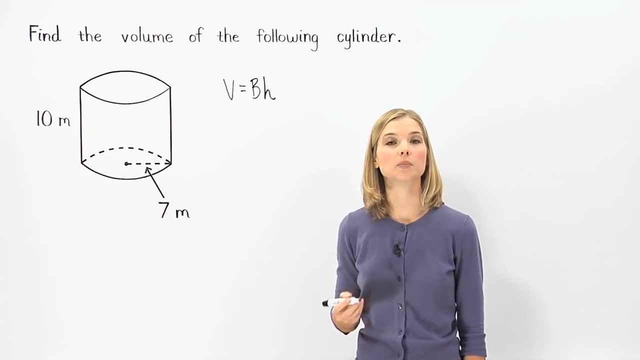 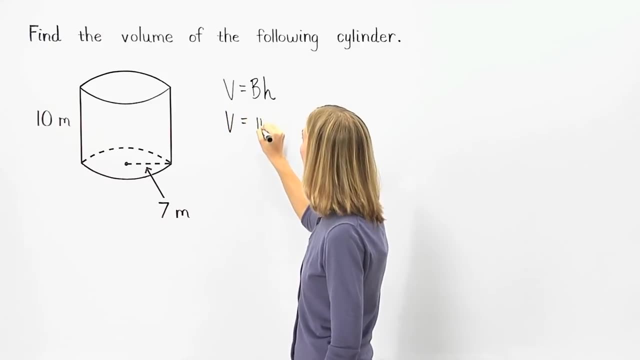 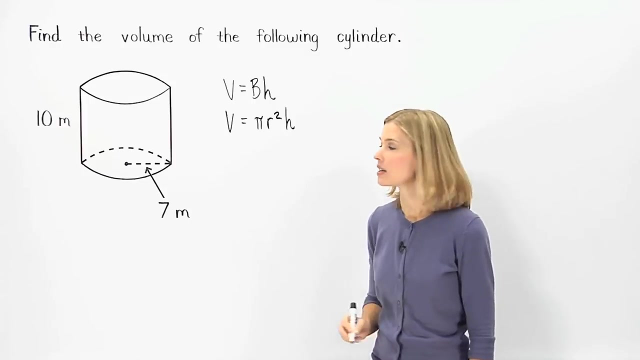 and remember that the formula for the area of a circle is pi times radius squared. So the formula for the volume of a cylinder can be written as pi times radius squared times height. So to find the volume of the given cylinder, since the radius is 7 meters and the height is 10 meters. 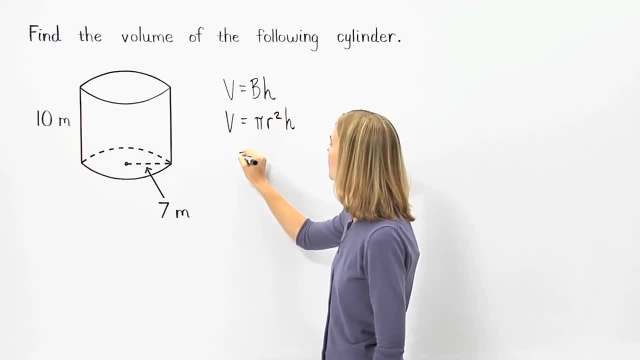 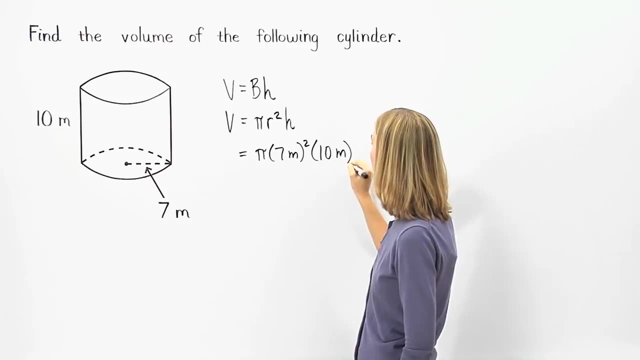 we can plug this information into the formula to get pi times 7 meters squared times 10 meters. Remember that 7 meters squared is the same thing as 7 meters times 7 meters, which equals 49 meters squared, And we have pi times 49 meters squared times 10 meters. 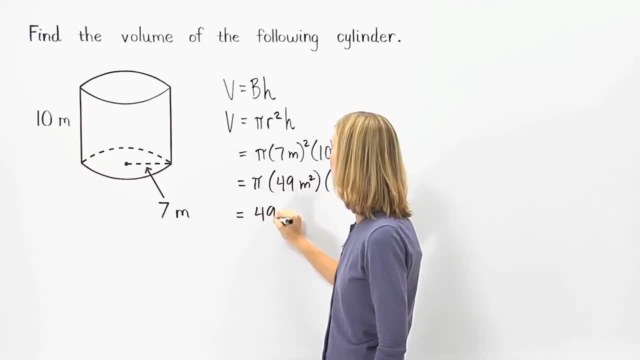 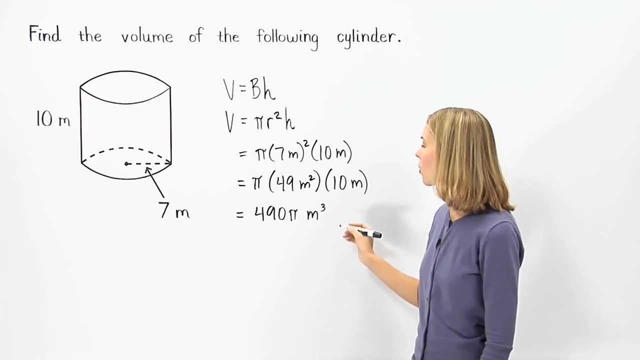 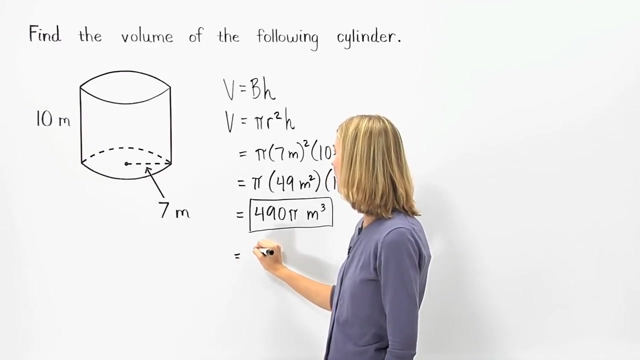 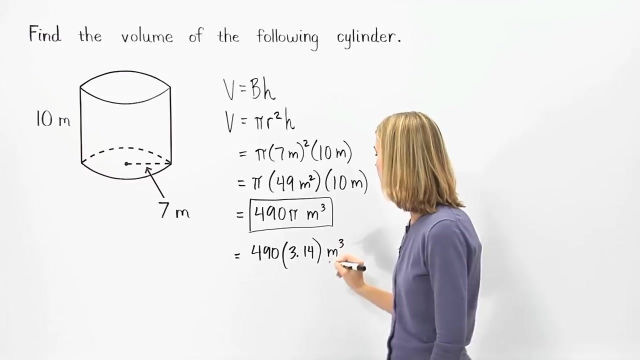 which simplifies to 490 pi meters cubed. So one way to write the volume of the given cylinder is 490 pi cubic meters. Next, remember that pi is approximately equal to 3.14.. So we can plug 3.14 in for pi and we have 490 times 3.14 meters cubed. 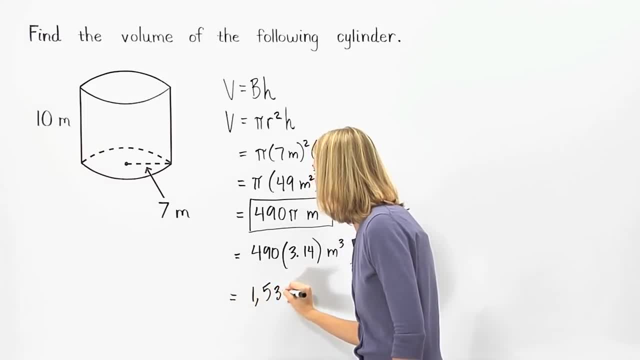 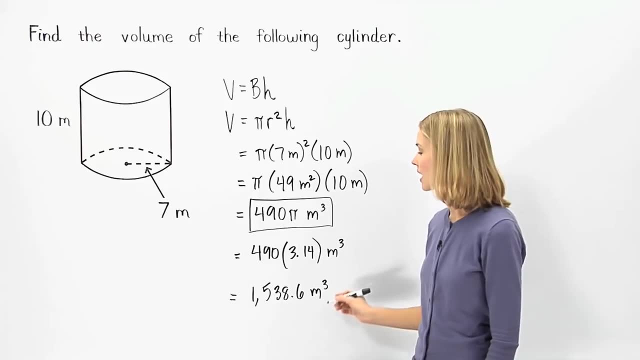 which equals 1,538.6 meters cubed. So another way to write the volume of the given cylinder is 1,538.6 cubic meters. So again for the volume of a cylinder, we can plug 490 pi squared times 6 meters squared.